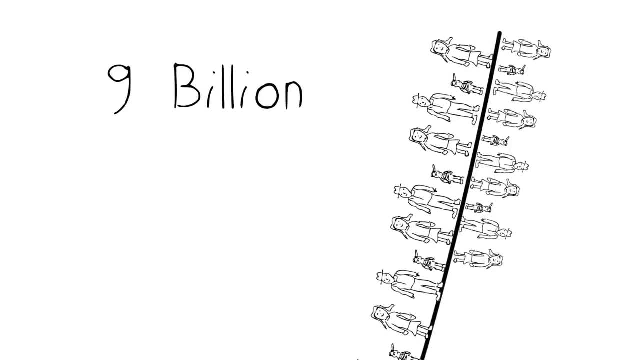 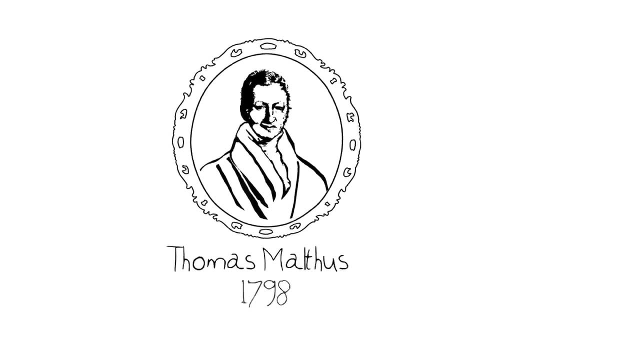 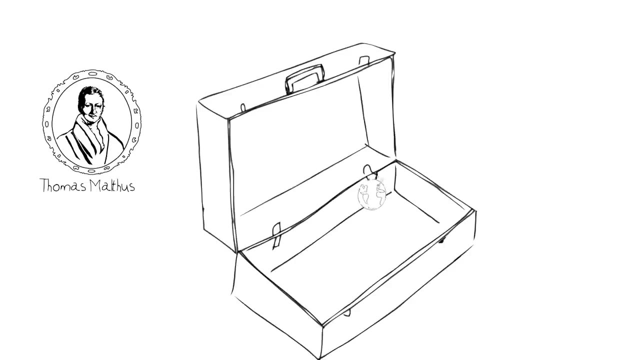 steeper to the point where we're looking at about 9 billion people by the year 2050.. It was Thomas Malthus in 1798 who came up with the concept of carrying capacity. Basically, he said that the earth can't indefinitely support an ever-increasing. 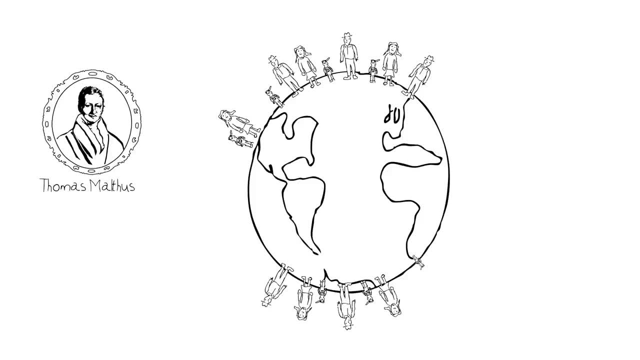 human population. That's a concept that to us, I think, seems quite clear. But Malthus was a member of a social force at that time, Basically the clergy, that felt the earth was put here for humans to use and upon which we should go forth and multiply. But Malthus was among the first in 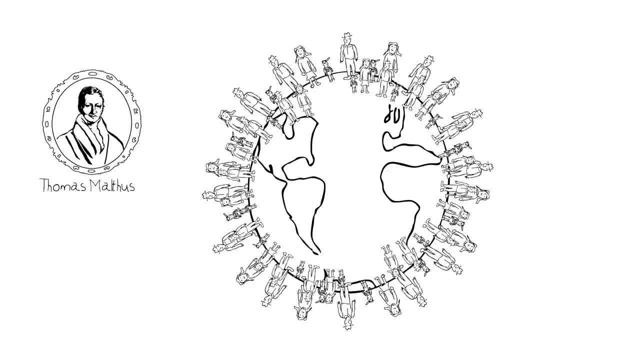 recognizing that there was no way that human population could increase indefinitely without having some sort of an effect on the environment and the environment's ability to support us. The logic he used led him to the fact that, based on the kind of farming he saw around him at the 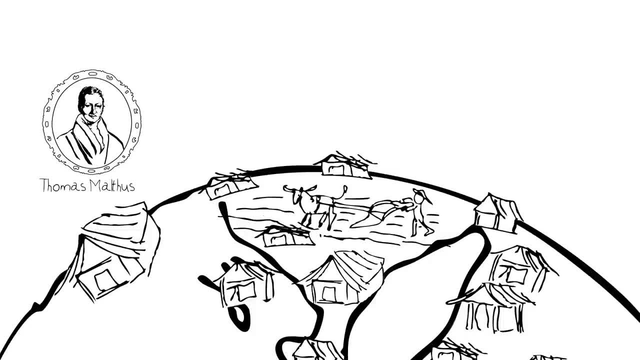 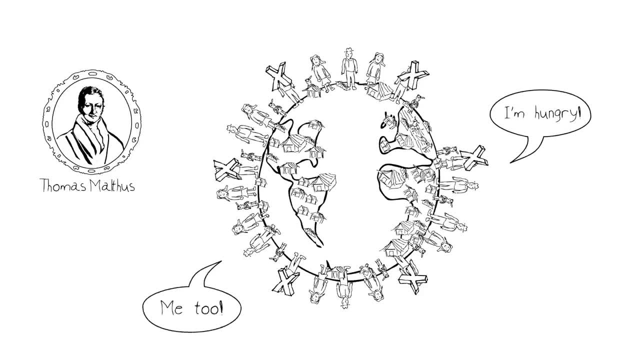 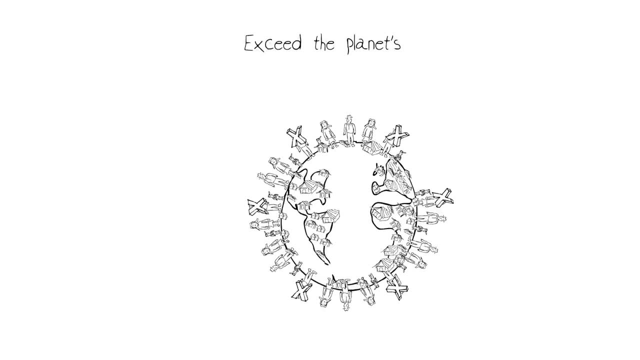 time, there would soon be so many people there wouldn't be enough to eat. Basically, the planet was going to check population growth through famine. He had seen famine, He knew what it was like, So the planet was going to take care of it. if we didn't, In other words, we would exceed the 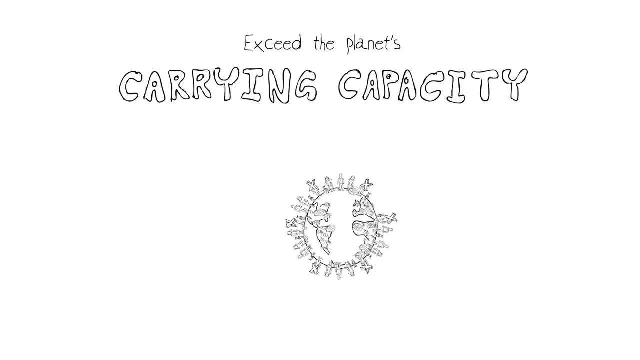 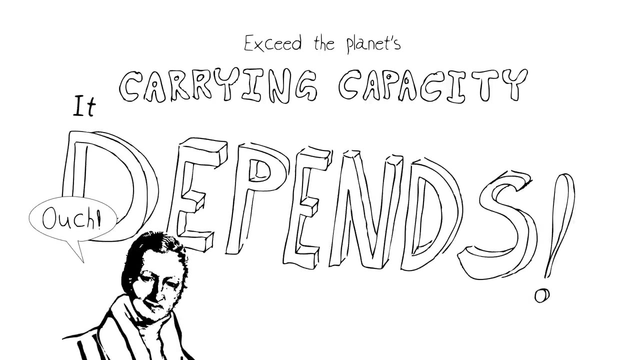 planet's carrying capacity for human beings. The question arose: what actually is the carrying capacity of planet earth for humans? The answer is, like most scientific replies, it depends. We haven't hit the Malthusian limit yet because of a very important thing, and that's human technology. 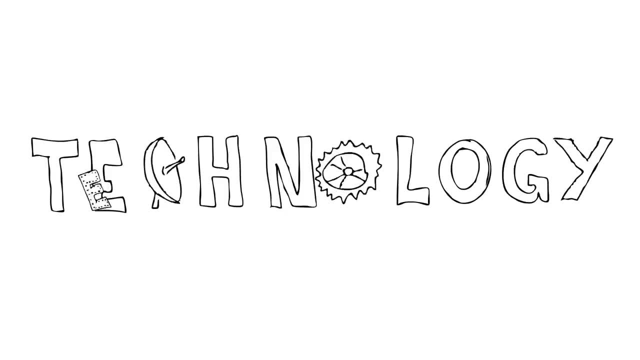 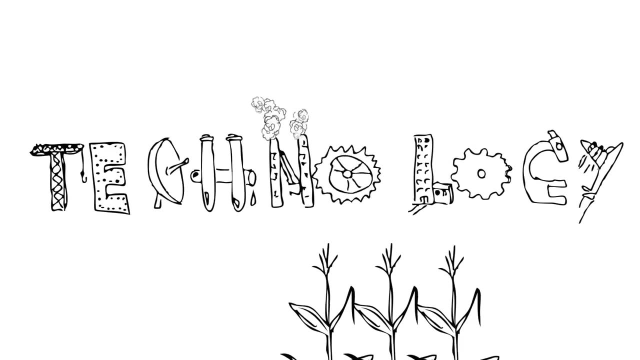 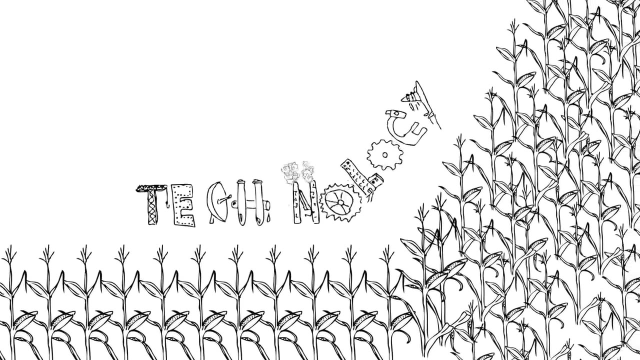 The ability to come up with answers to problems that are facing us at almost every turn. In this case, the answers came through science and technology. This made it possible for us to get back on the exponential population growth curve and escape Malthus's view of what the upper limits were. In fact, there are some estimates that suggest, if we 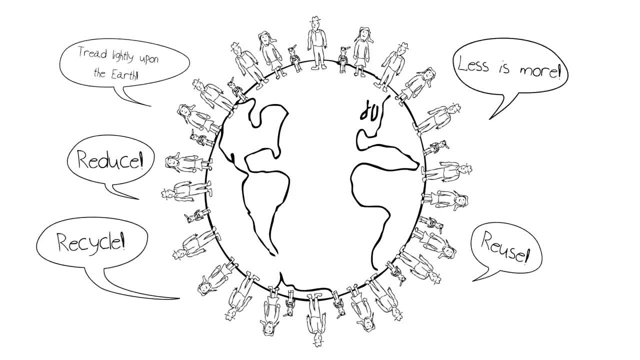 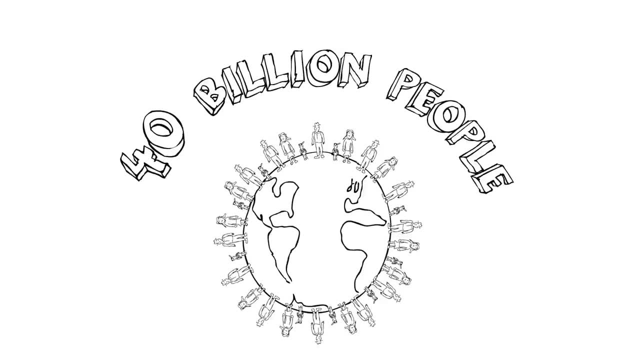 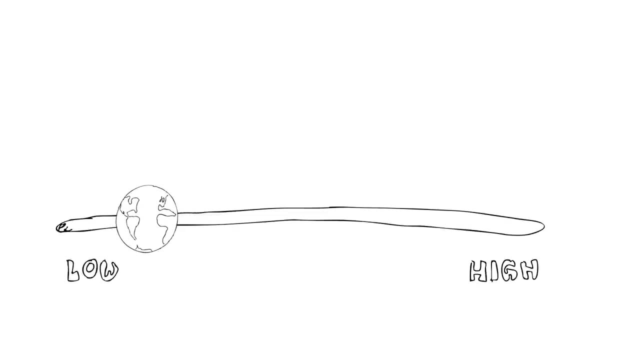 all did with less and lived at the lowest possible level for existence. earth could support an estimated 40 billion people, But even if we were able to reach a carrying capacity of 40 billion, it would require sacrifices for all humans on earth, Some more than others. it raises a huge question about the quality of life, which points out what's 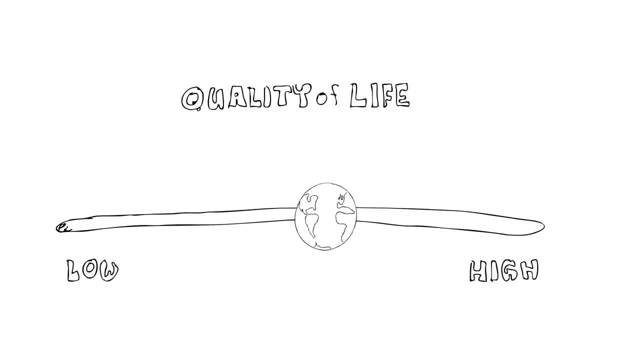 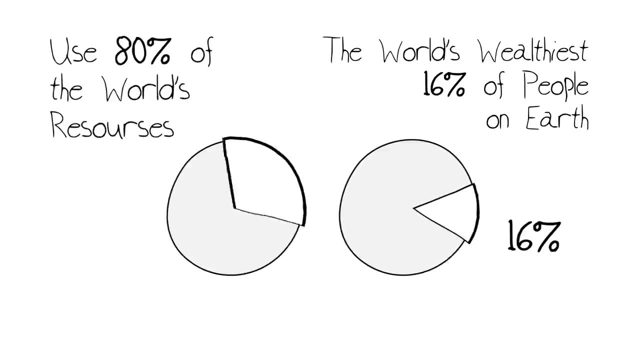 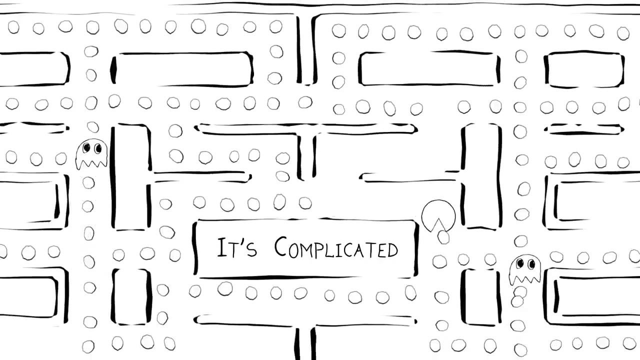 increasingly becoming the single most important fact about human population growth on earth today that the world's wealthiest 16% of the people on earth use 80% of the available resources. The bottom line here, as I say, is that it's complicated. We recognize that the human 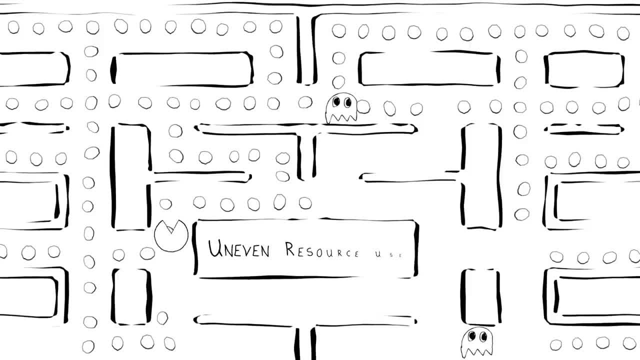 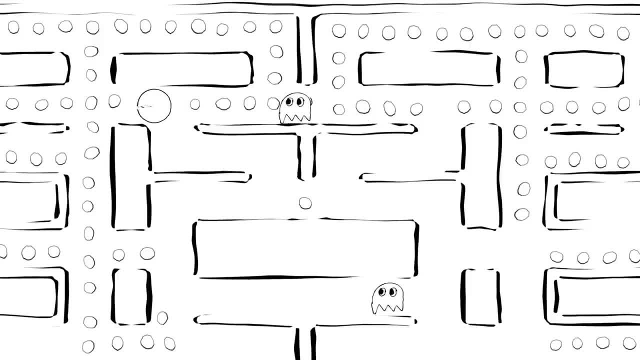 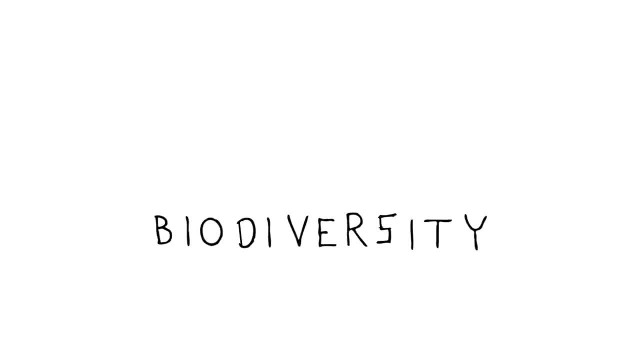 But what I really want to do is circle back to our primary objective and examine what this really means for biodiversity. If you asked anyone, they'd say it's pretty clear that human population growth and resource utilization have huge effects, not just on our social and economic well-being. 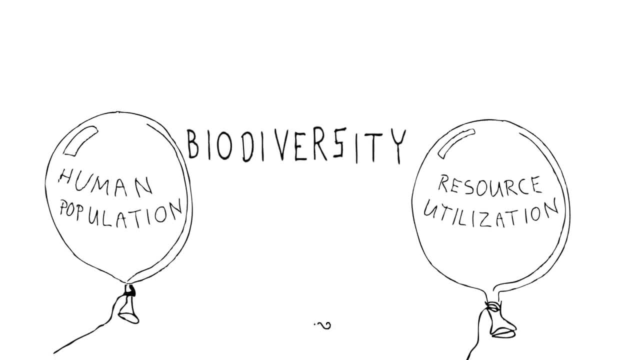 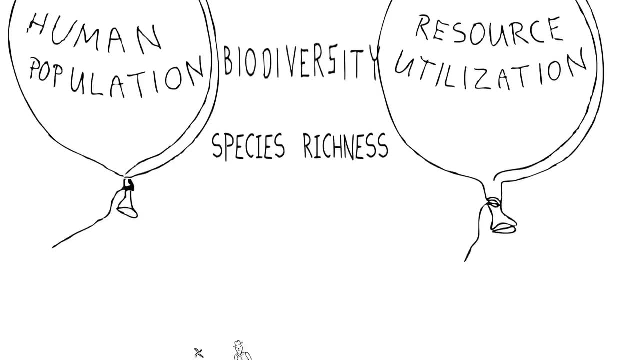 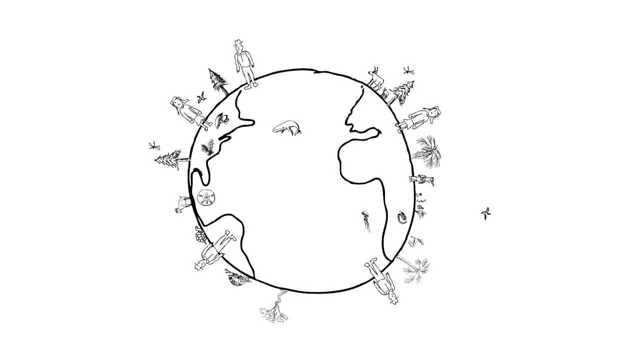 but of course on biodiversity. But how exactly It translates into decreases in species richness? It's primarily through the loss of species richness that our greatest population growth effects are going to show up. If we simplify it, it's as fundamental as no two things can occupy. 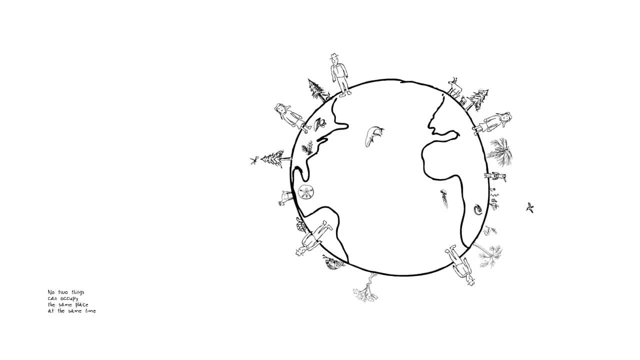 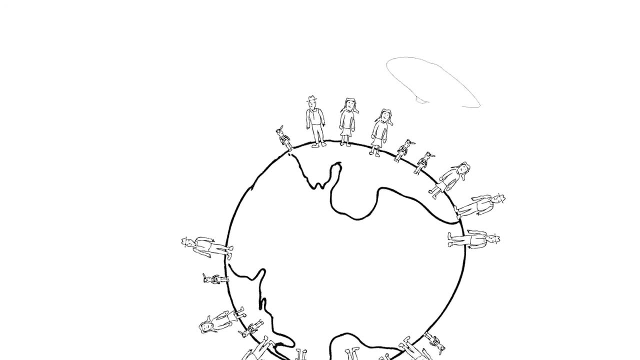 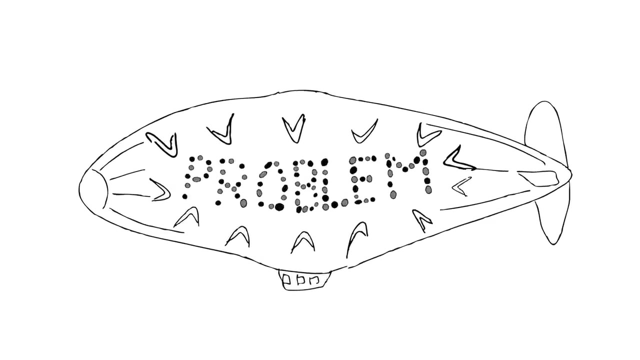 the same place at the same time. That's what we're talking about. If a human is living in a given place, fewer native plants and animals can live there. The details of how human population growth actually affects species richness are only now starting to be worked out. We don't have a lot of data yet. It's a huge complex. 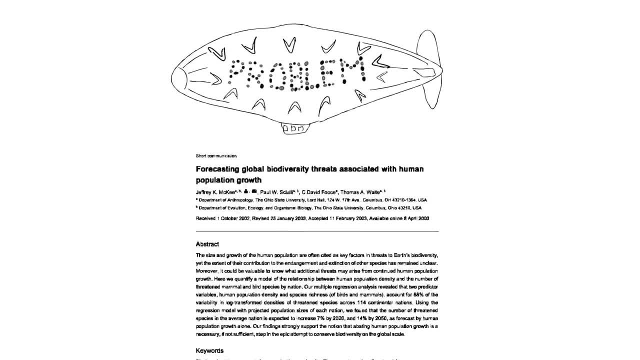 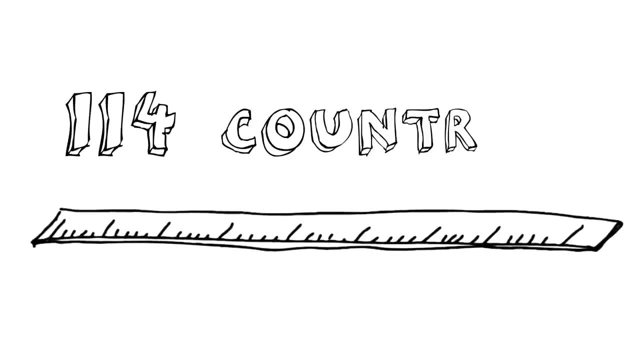 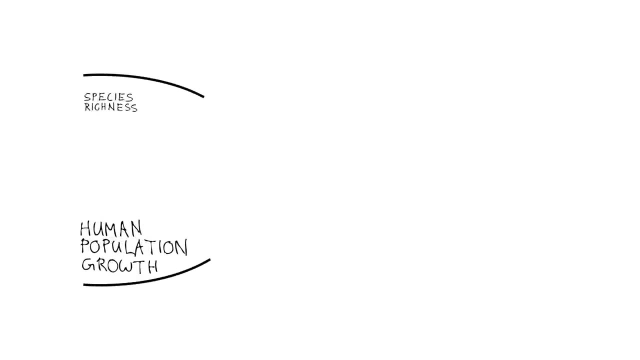 problem. One of the pioneering papers on this was published in 2003 by McKee and colleagues. They measured a number of factors in 114 different countries and what they discovered was that, out of all the factors that they looked at, human population growth and species richness- 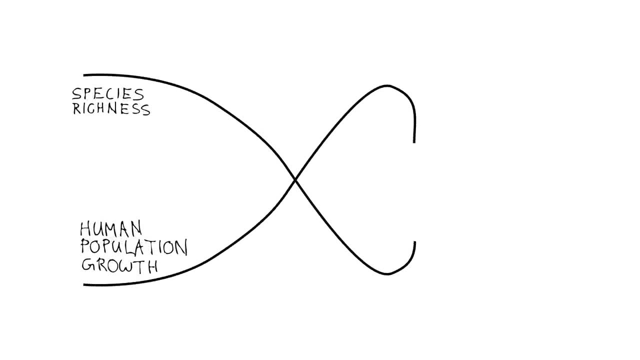 were tightly linked. In other words, if you were to slow population growth, that might be sufficient to stop drops in species richness. They suggested that we could take a look at the results of the study and see what we could do. They suggested that we could take a look at the results of the study and see what we could do. 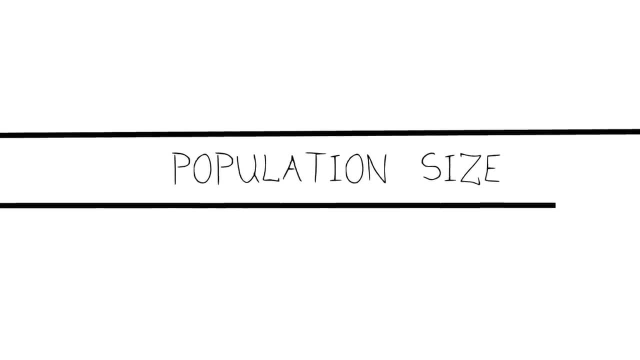 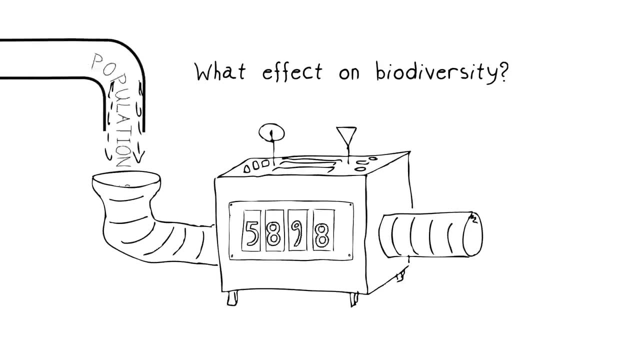 that all you need to know is population size. Plug this into the equation and you can figure out in a given place what effect it's going to have on biodiversity. Calculations show that the number of threatened species in an average nation is going to increase 7% by 2020 and 14% by 2050. 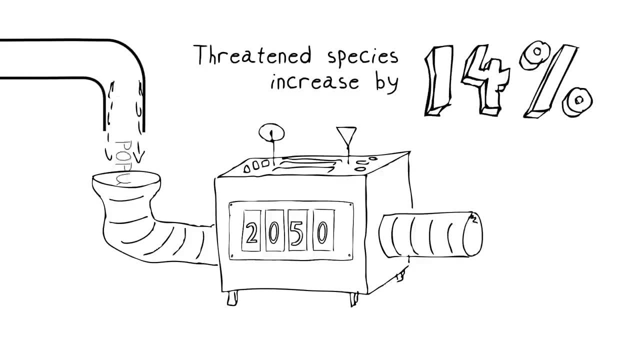 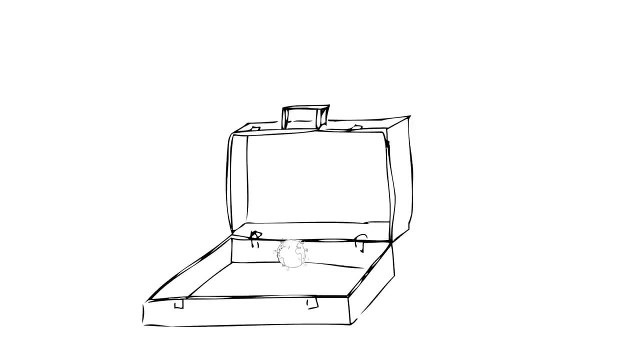 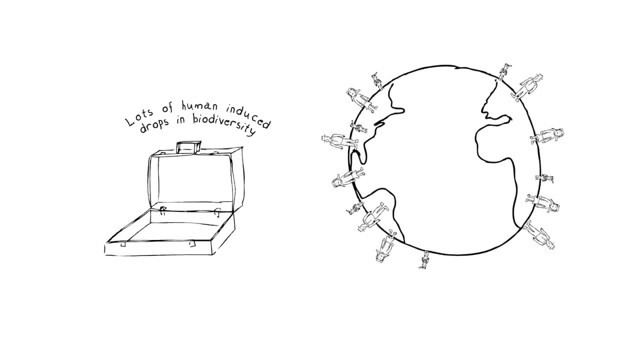 just based on population growth alone. That's a very simple relationship, but if you open up that box represented by the idea of population growth and unpack what it means, you're talking about lots of human-induced drops in biodiversity And, as usual, things get complicated. I'd say that there. 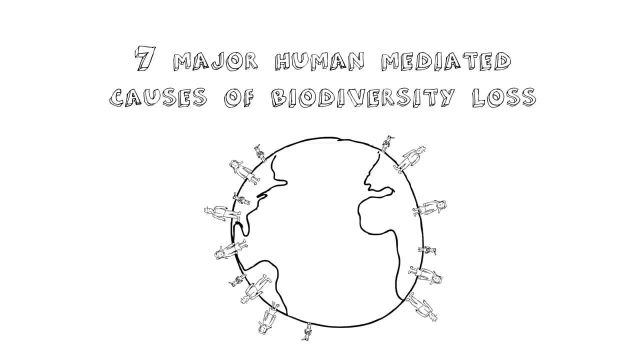 are seven major human-mediated causes of biodiversity loss. They can be grouped into two main categories: localized ones and global ones. The global causes we'll look at in separate videos, but for the localized ones, we're going to talk about the two main categories: localized ones and global ones. 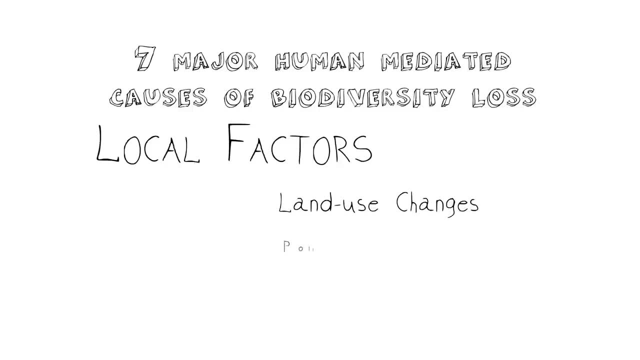 On the list four: land use change, pollution, resource exploitation and introduction of exotic species. Of course they overlap a little, but I think for the most part these are good ways of unpacking our box of problems. Let's start with land use changes. These include things like 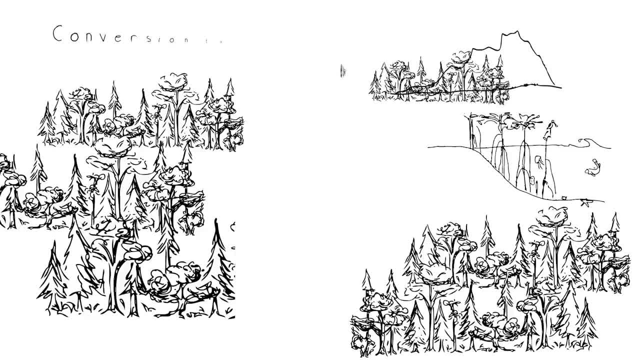 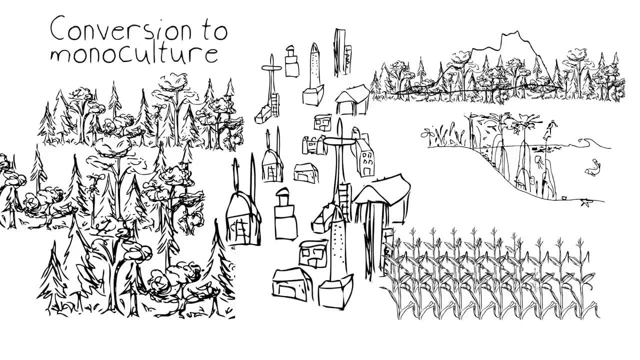 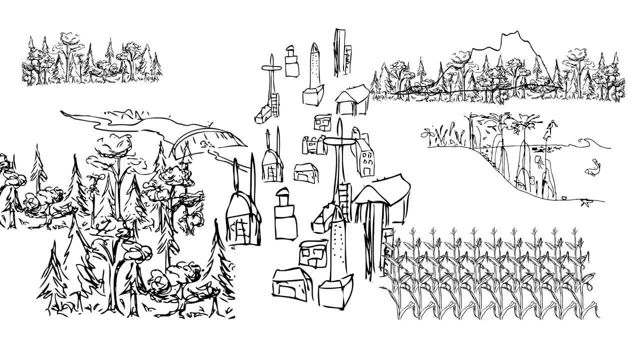 habitat destruction and conversion of natural habitat to human use that isn't necessarily compatible with the organisms that are native there. This includes crop monoculture that results in a very dramatic drop in species richness in a given habitat. When people think about habitat destruction and conversion, they think of 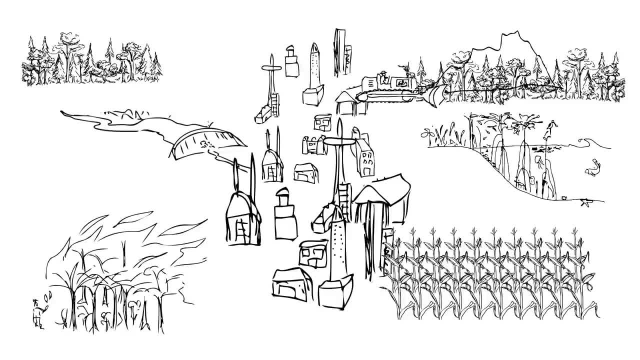 slash and burn agriculture, destroying rainforests, plowing overstuff or removing the tops of mountains to get at resources like coal. But there are ocean use changes too that I think we should not ignore. Think of coastal wetland loss and mangrove destruction. 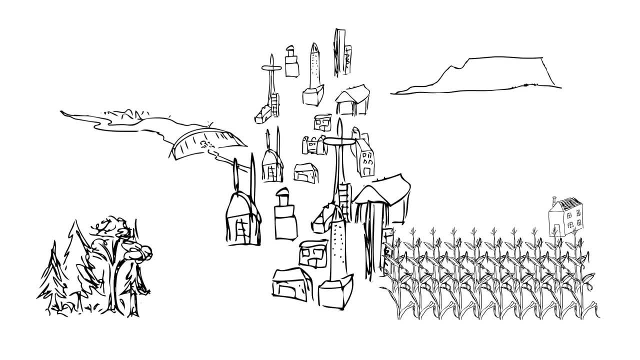 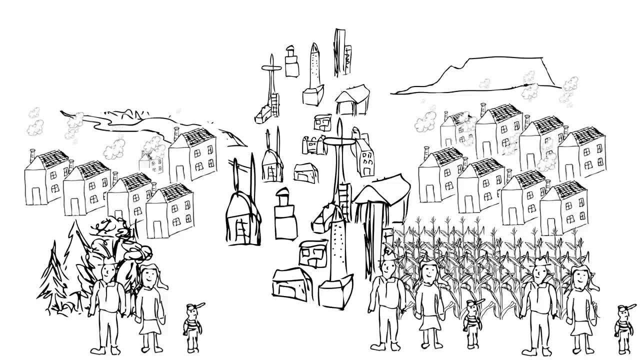 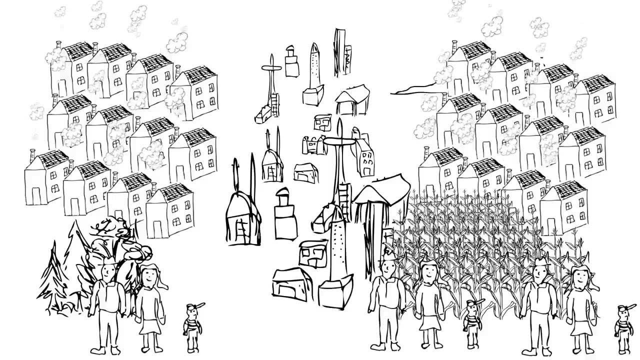 Urbanization is an enormous change in land use. More people need more homes and more places to work. That, in turn, requires an expansion of agricultural resources and the spread of those into environments that were previously untouched. It's a very complex problem, as I say, but simply. 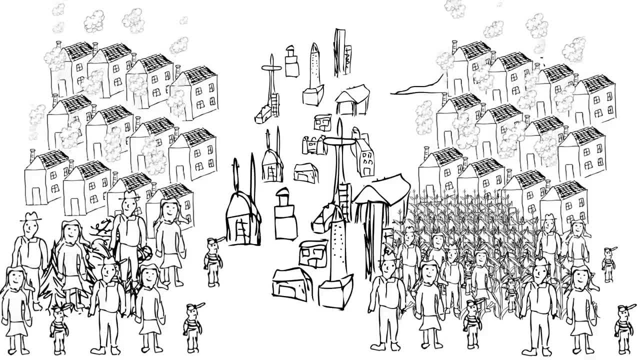 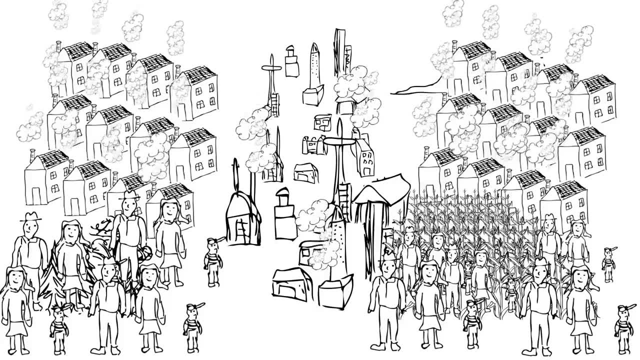 put, the more people you have, the less natural undeveloped habitat there's going to be, And it's very easy to see how that's linked to a drop in biodiversity. The second local factor is pollution. A lot have been done to bring this subject to people's. 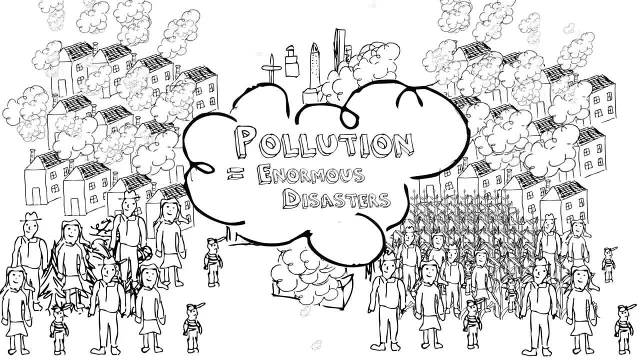 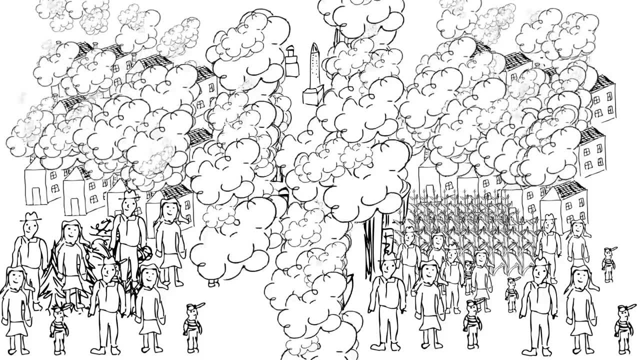 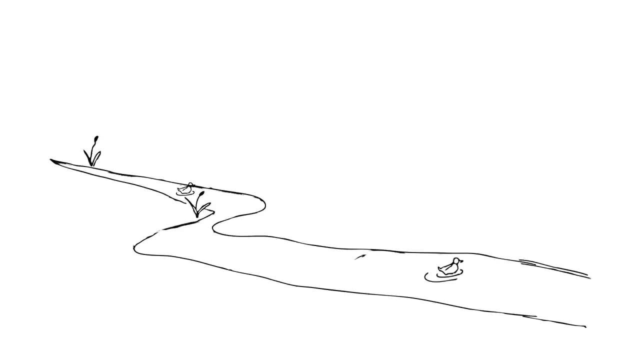 attention to the point where we think about it as enormous disasters attached to super fun cleanup sites and such. But there are other, more subtle ways of polluting the environment which I think are worth thinking about. when we talk about drops in biodiversity, For example, the degradation of 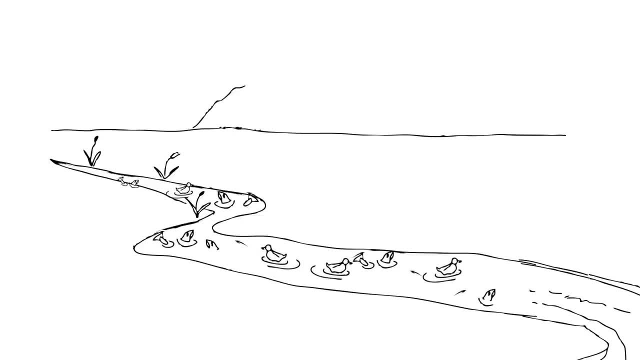 local habitats through human activities that cause downstream effects, Things like the leaching of harmful chemicals from mines into the water table. Waterborne pollutants can pop out in very unusual places and have really big downstream effects. if you'll excuse the pun on the 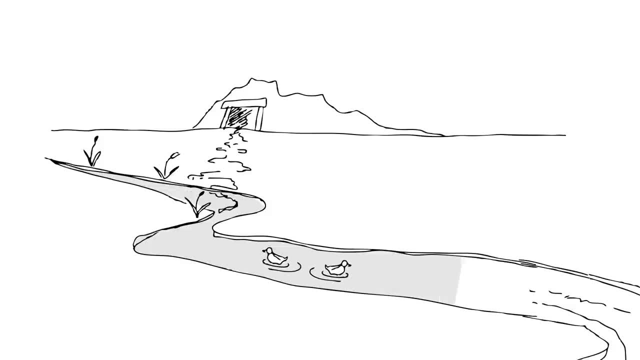 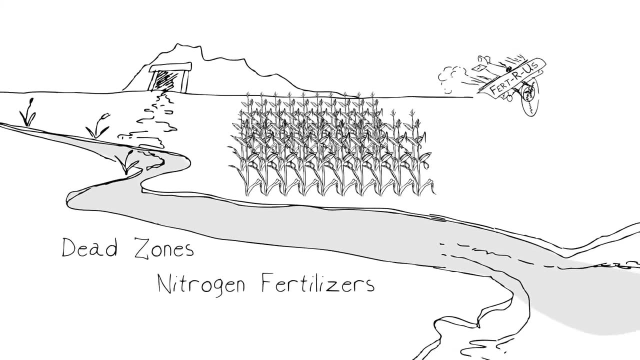 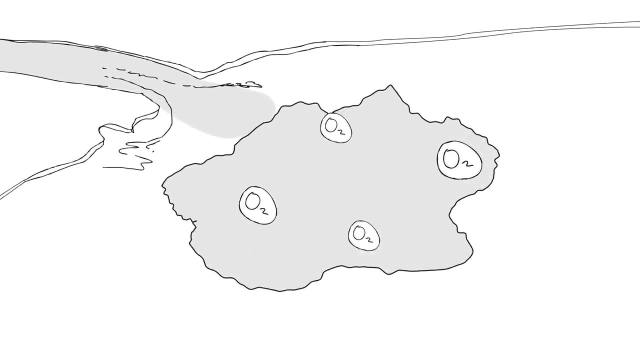 reproductive viability of organisms that happen to be in those places. There are also dead zones in the ocean caused by nitrogen fertilizers that wash into rivers. Where the rivers flow into the sea, the nitrogen causes blooms of bacteria, which in turn use up the oxygen. 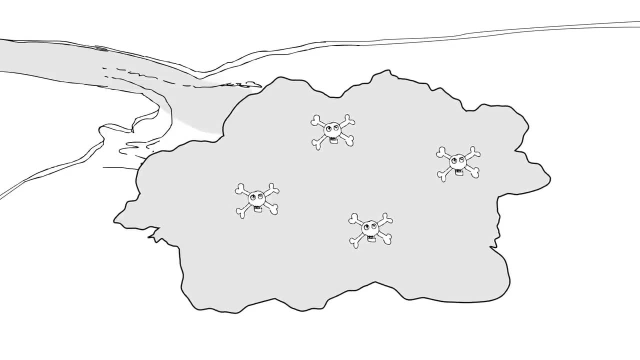 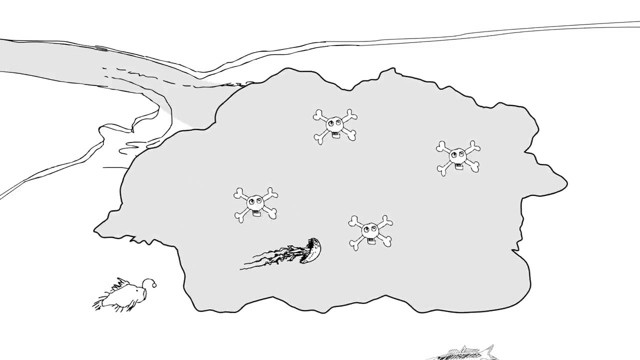 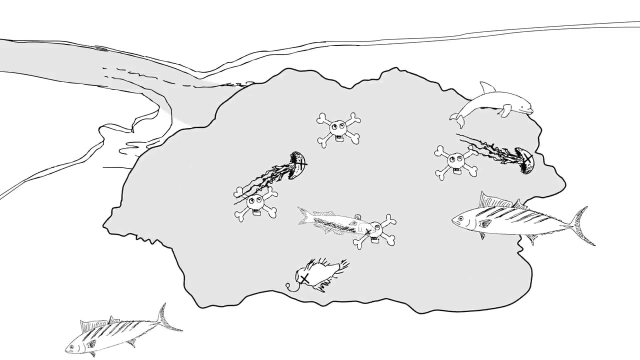 Anything that tries to be active in an area where the oxygen is being used up by the bacteria. any oxygen-requiring organism- that is, pretty much any animal, for example- is going to have a really hard time of it. These dead zones are now starting to be a little bit better understood, and it's 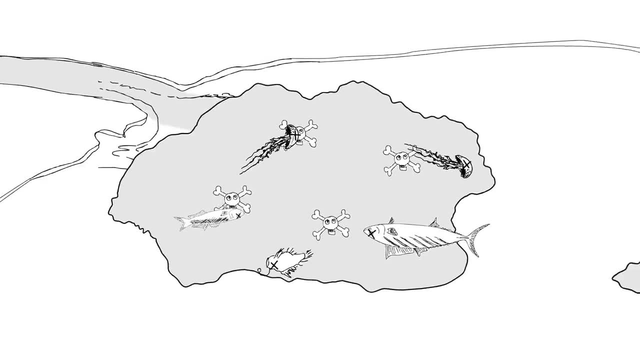 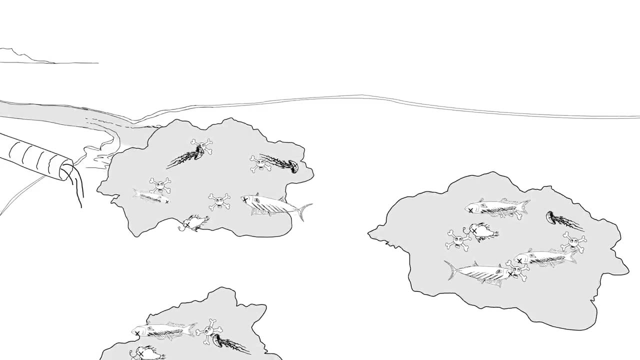 pretty clear that they're growing in size and in number in relation to population growth. Then there's the overall problem of waste disposal. Untreated sewage is a classic problem for biodiversity. It's not just, of course, human waste It has to do with, sometimes bizarre chemistry involved in the high-tech stuff that we're making. now. We're talking about chemical compounds, including drugs and PCBs. There are lots of strange molecules that humans are producing and dumping. In some cases you get these hormone mimics- simple compounds derived from. 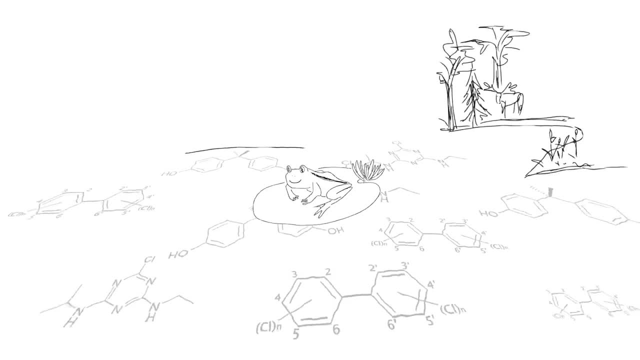 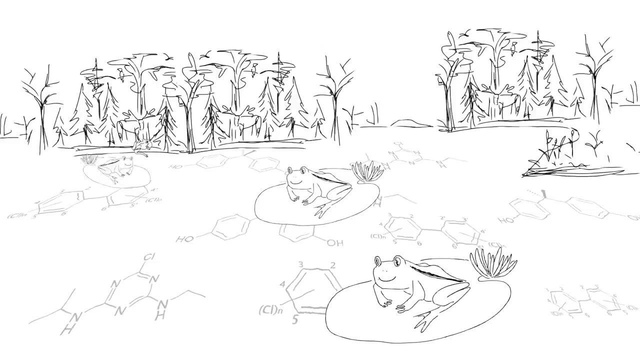 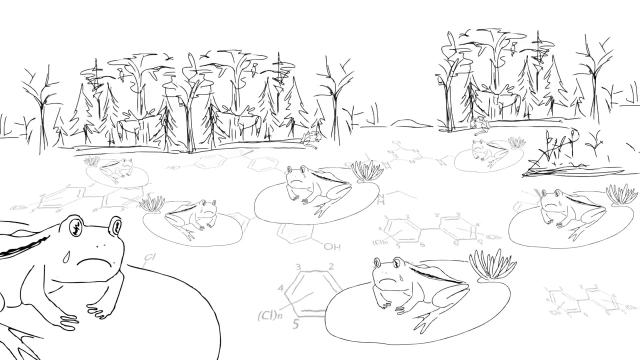 prescription drugs and other man-made chemicals that get flushed into waterways. Hormone mimics act like naturally occurring hormones that control normal development in wild organisms, particularly water-living ones. Hormone mimics can also adversely affect their reproductive organs, and there are many, many, many examples of this kind of pollution, one that people wouldn't 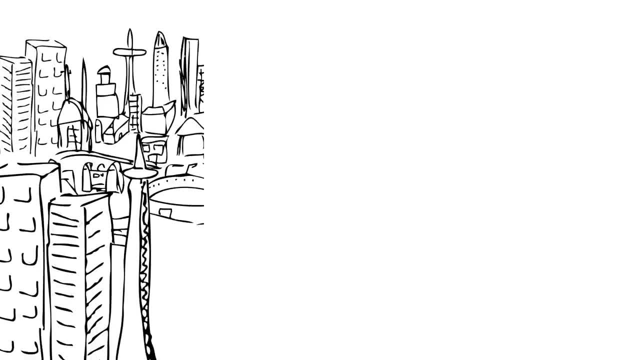 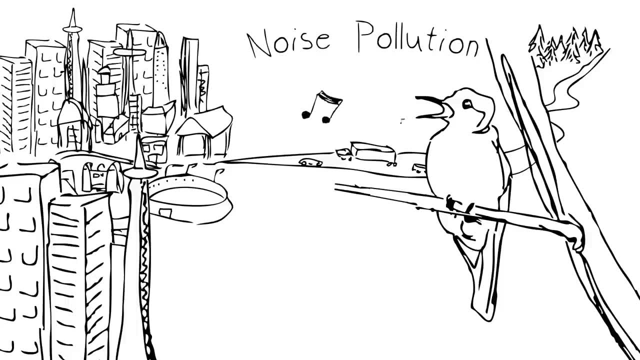 necessarily think of. Another one that doesn't immediately occur to people is noise pollution. Birds and cities are reacting to noise levels, so even the organisms that are not being wiped out because of our expanding cities are starting to adapt to an urban environment by changing their behavior and reproductive patterns, And some of them just can't do it. 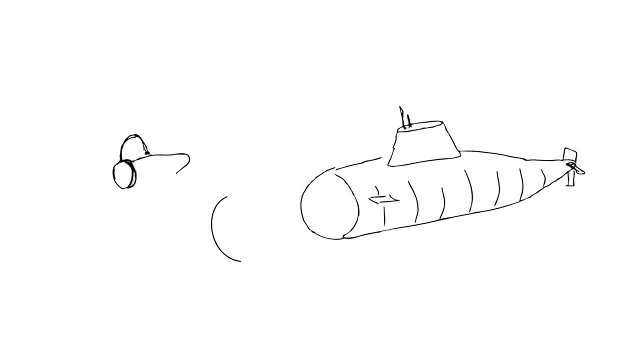 Noise can also be a major factor in marine mammal survival. Evidence suggests that sonar pollution interferes with the health of marine mammals. Patterns of reproduction can also be upset by our introduction of light pollution to places where there wasn't light before. Sea turtle hatchlings can be impacted by artificial light heading toward it instead. 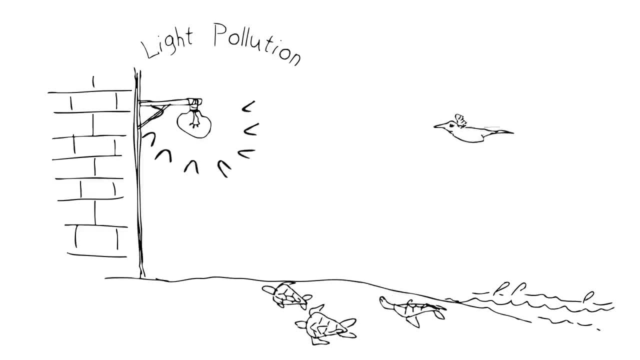 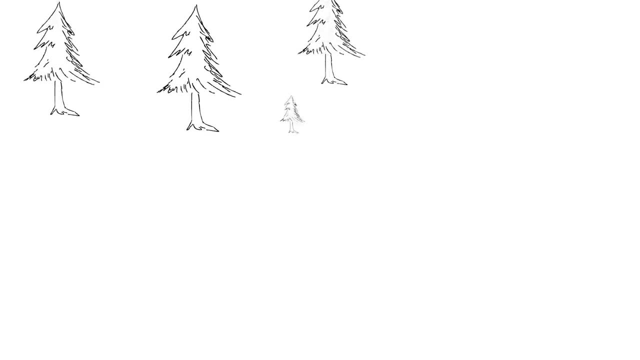 of the ocean when they hatch out of their nests on the beach, And bird strikes on buildings are greatly increased at night, when the lights are left on. Let's look at the third local factor: resource exploitation. This gets to the simple idea that humans are always using things from. 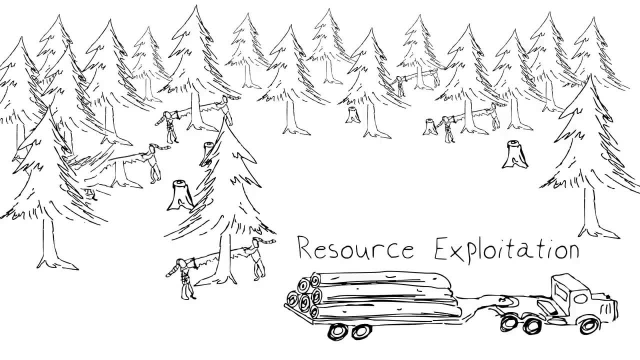 their environment. We are inextricably linked to that environment and we use up stuff We always have. We have been called to watch the environment every day for years. We see the things we've learned. We have to do that in order to stay alive. 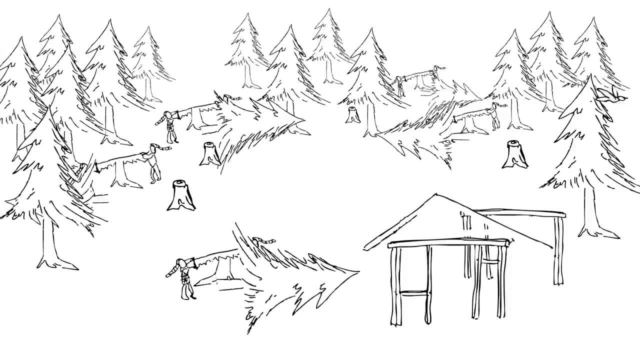 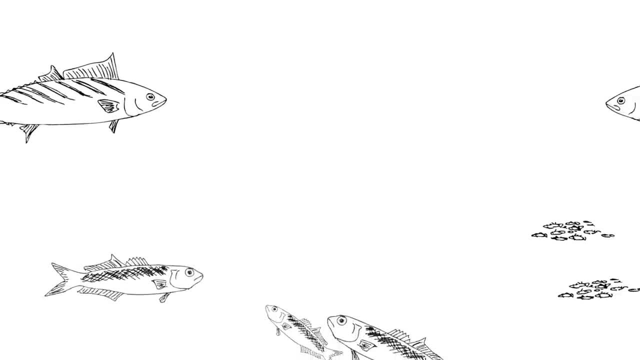 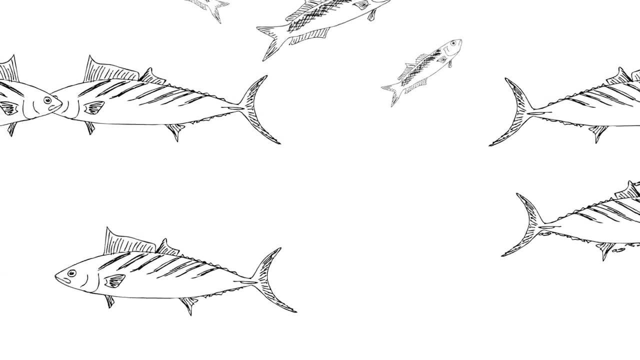 There are classic ways we use resources, like hunting, cutting down forests for firewood and lumber. Where does the biodiversity go, then? A big one for me as a marine scientist, of course, is fishing. We talk about the harvest of fish, but it's not really a gathering of what one sows. It's really a straight-up removal of a resource as much as mining is. There are attempts to control over fishing, but to a large extent we often don't have enough data to know just what a sustainable amount of extraction is, until it's too late. 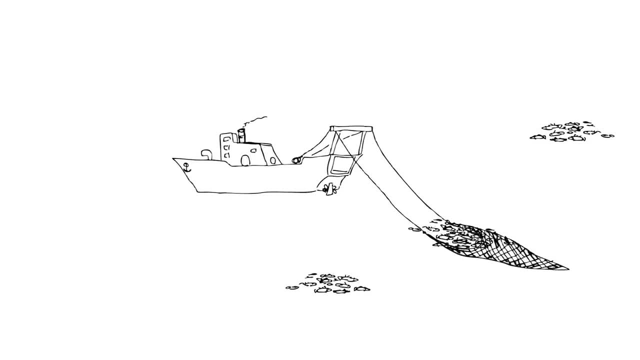 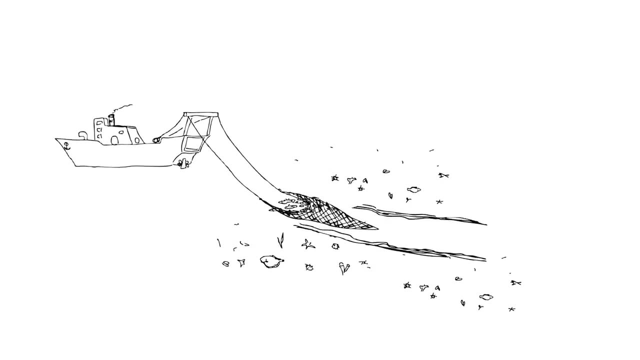 Before we were moved to action, for example, the cod fishery had collapsed on the Grand Banks of Newfoundland. Today we have no idea what the long-term effect of huge trawls scraping over the sea bottom will be. Now countries are pushing to fish more in the Antarctic. 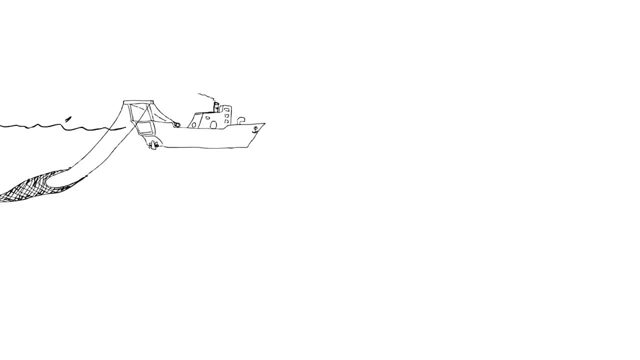 which is a problem because fish, like most things there, grow slowly in the cold Antarctic depths. The last local cause of reduction in species richness I want to mention is the introduction of exotic species, and we'll talk about those in the next video. 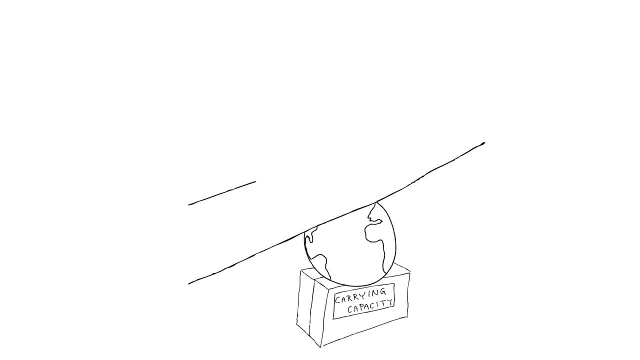 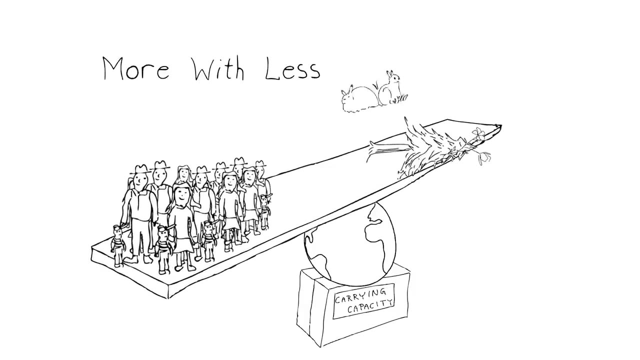 So, just to bring it all back to this concept of carrying capacity, the emerging message is that if everyone on Earth can manage to do more with less, especially in places where we presently use up relatively so much more, we might be on track to do more with less.